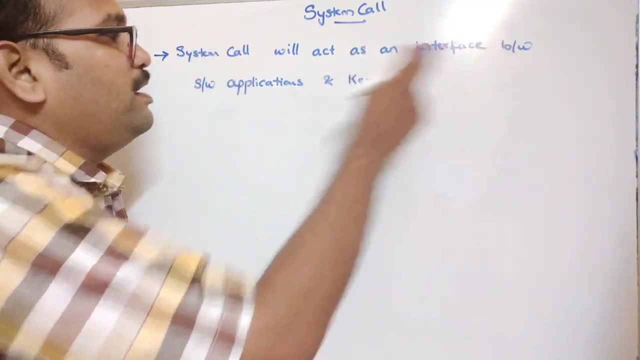 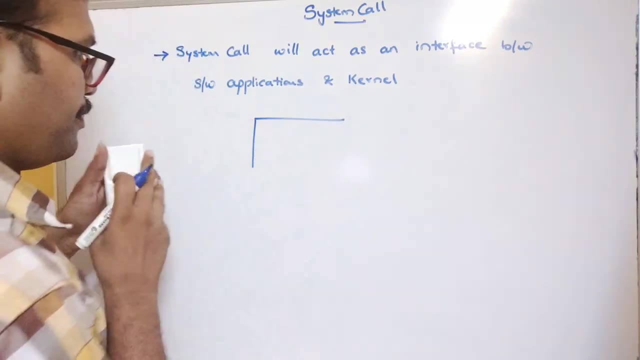 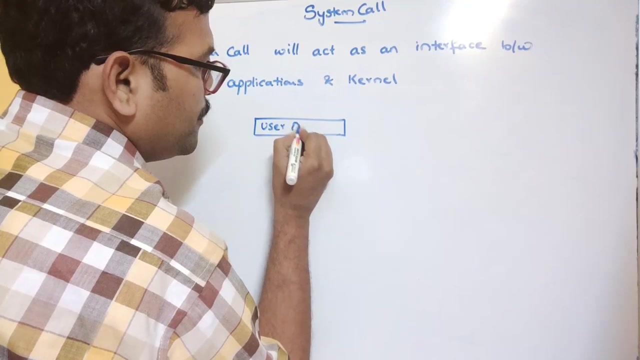 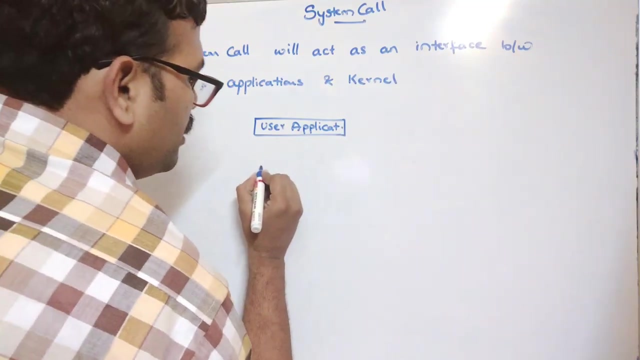 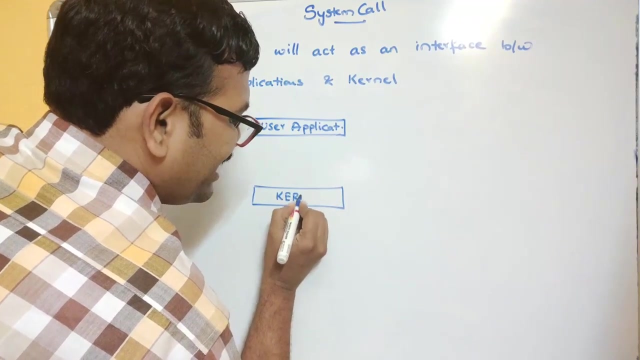 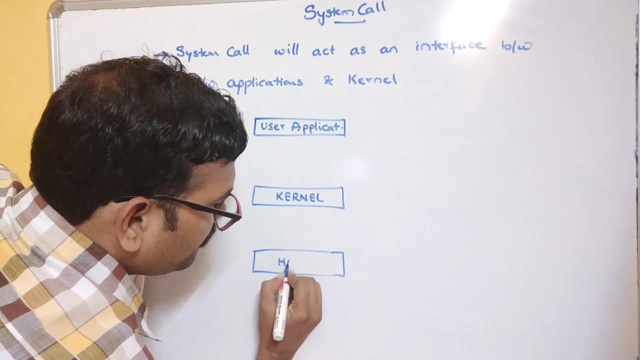 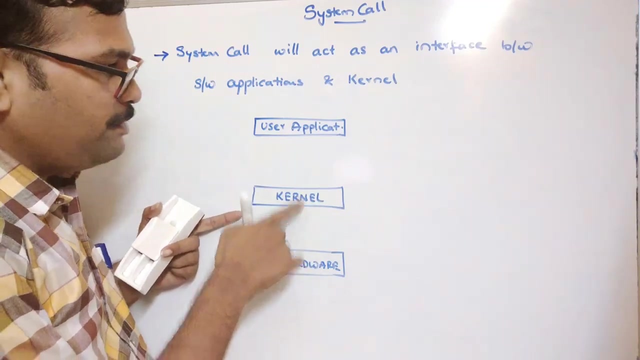 But here the system call is an interface between the applications and the kernel. So, if you observe, so these are the user applications And this is the kernel and this is the hardware. So this kernel will be acting as an interface between applications as well as the hardware. 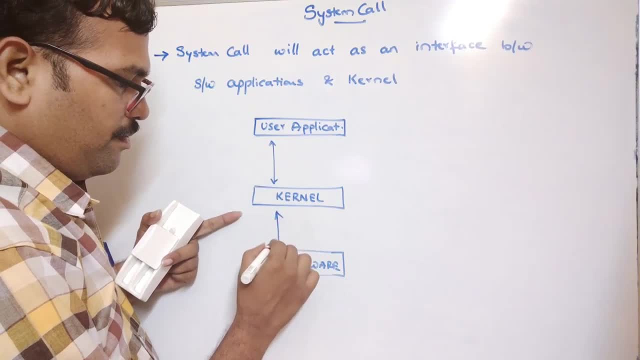 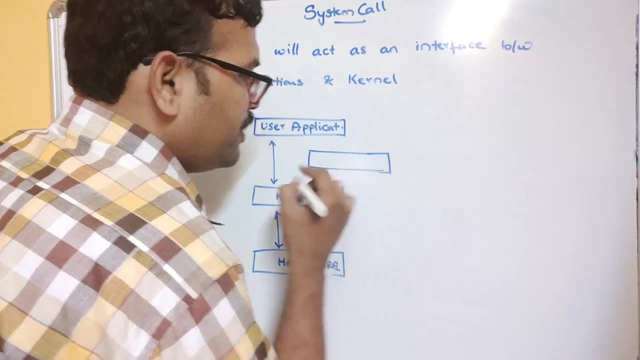 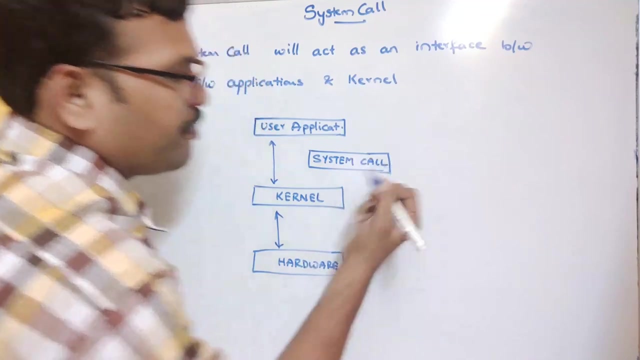 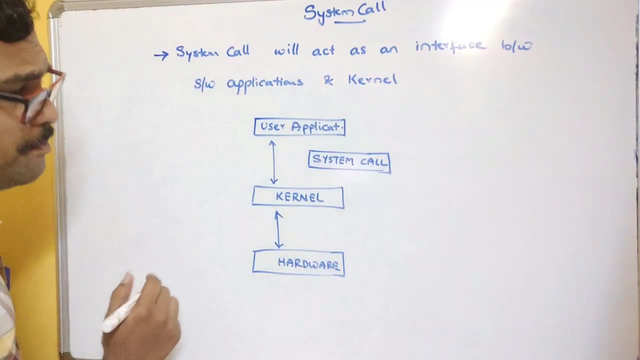 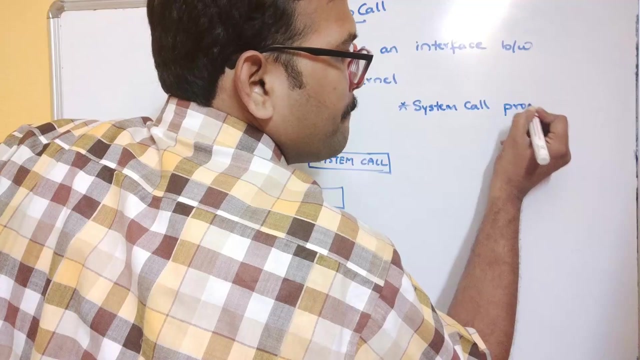 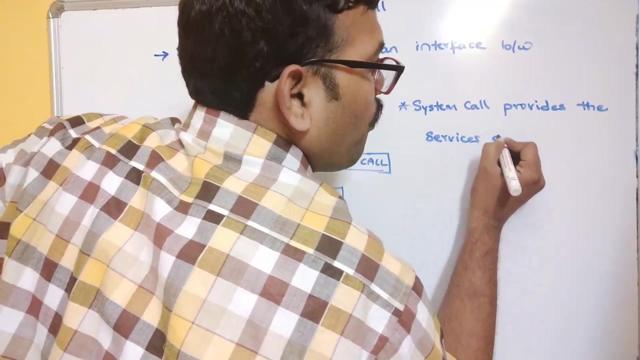 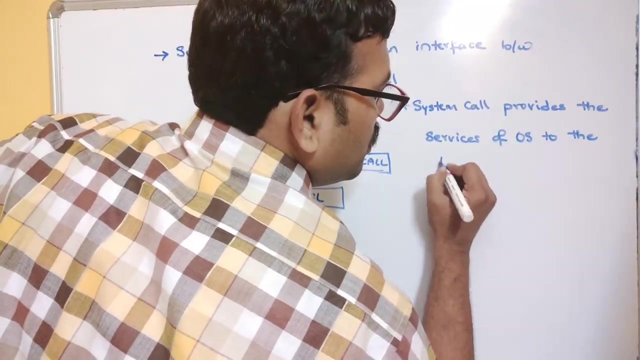 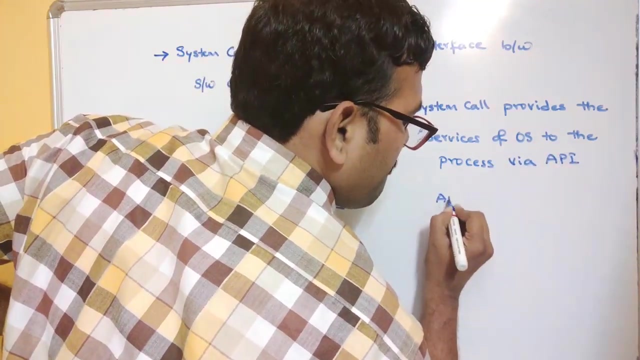 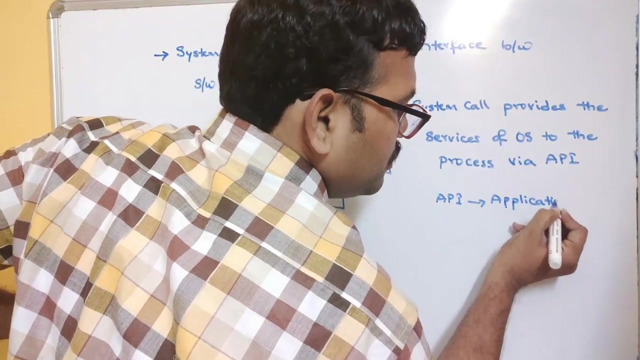 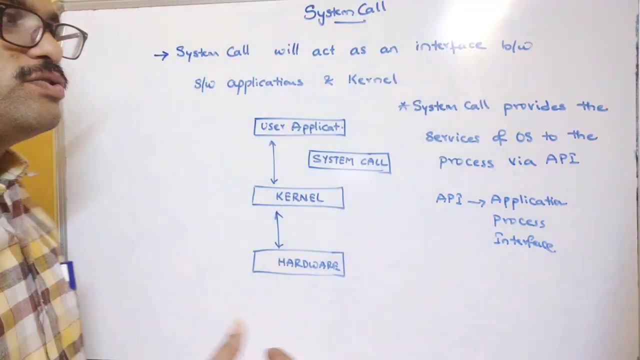 Now, this system call acts as an interface between applications and a kernel, And this system call provides the services of operating system to the process via API. API means Application Process Interface. So whatever the resources the process requires that will be provided by this system call. 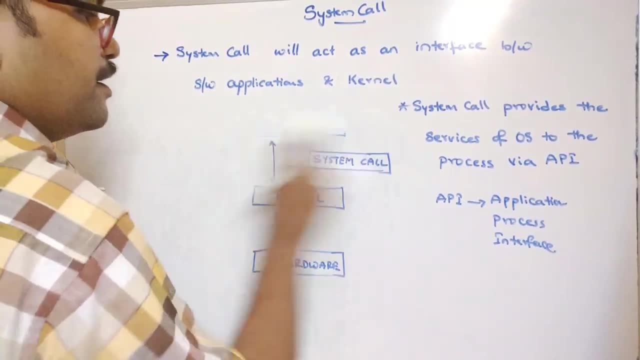 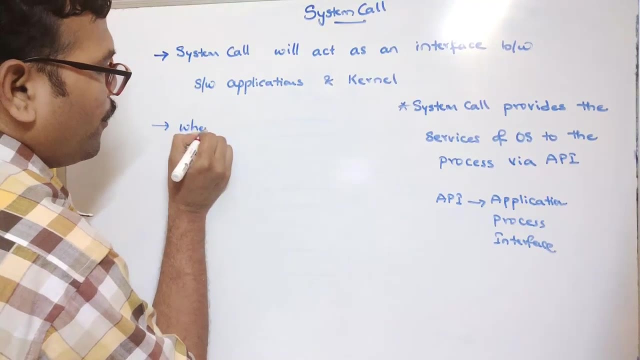 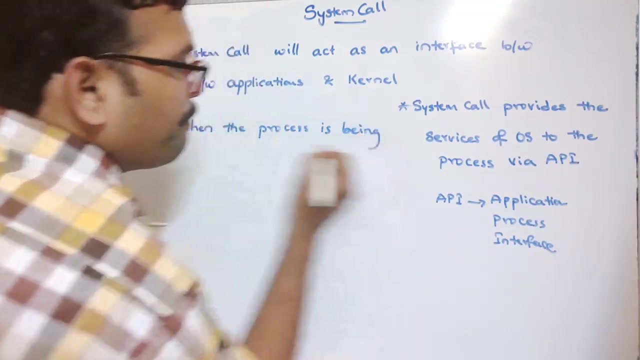 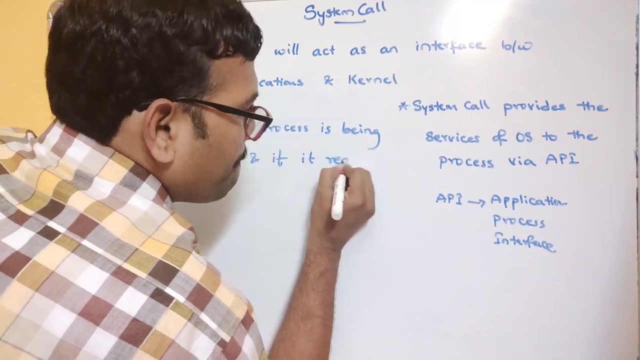 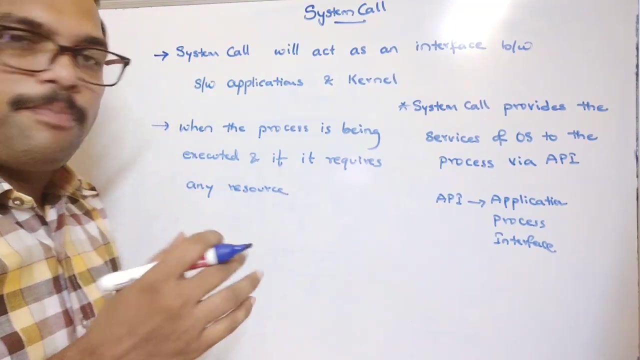 Right, So see, Whenever the user- I mean the process- is executed, when the process is being executed and if it requires, it requires any resource, any resource. Okay, So whenever the process is being executed, Sometimes it may require some resources. 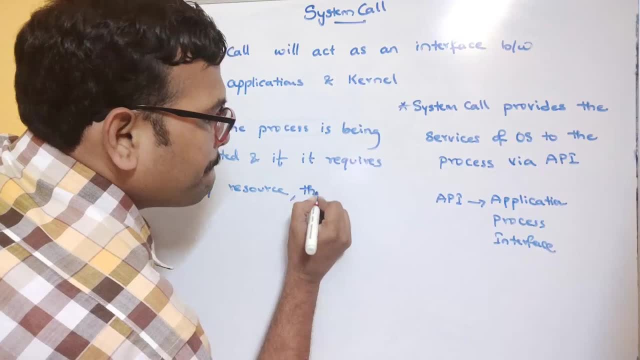 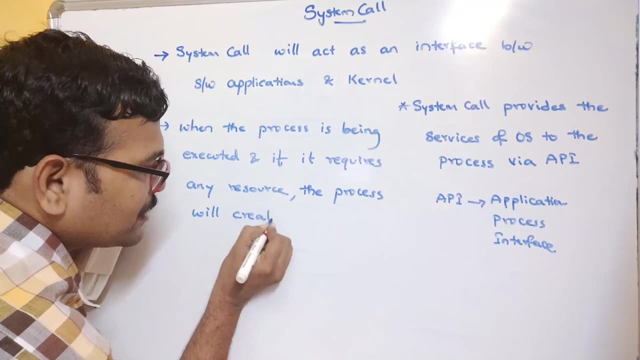 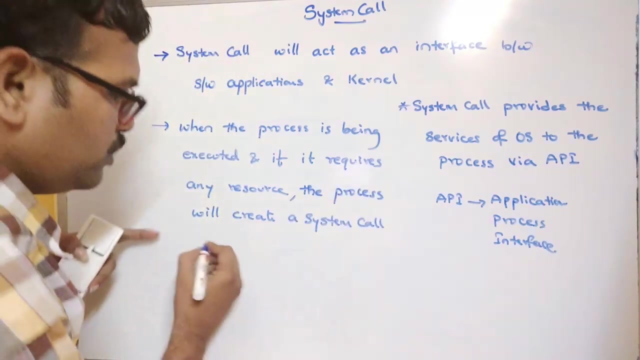 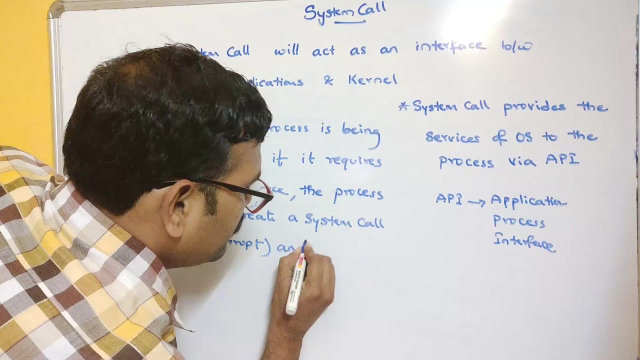 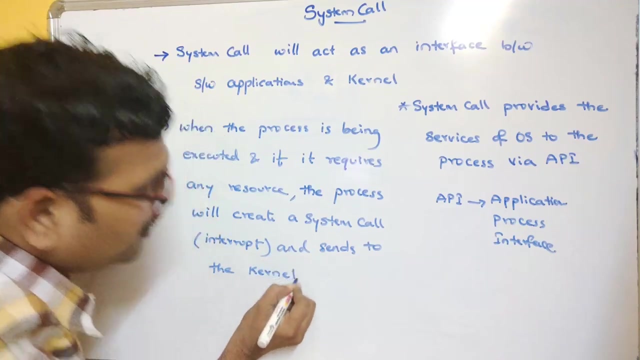 So whenever it requires any resource, then the process will create a system call. A system call, Okay, A system call which is nothing but interrupt, Interrupt Right And sends to the kernel. So here, whenever it requires any resource, then the process will create a system call. 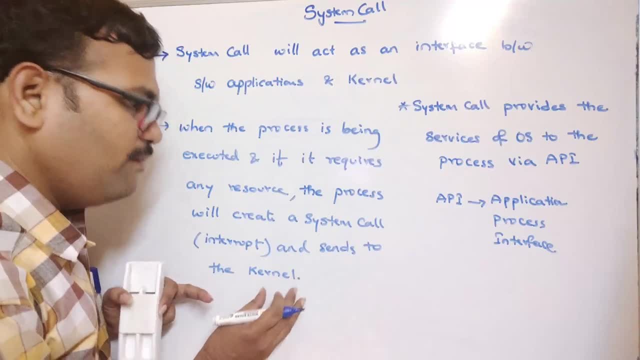 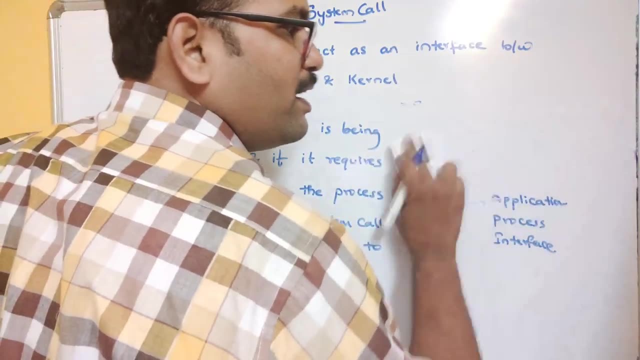 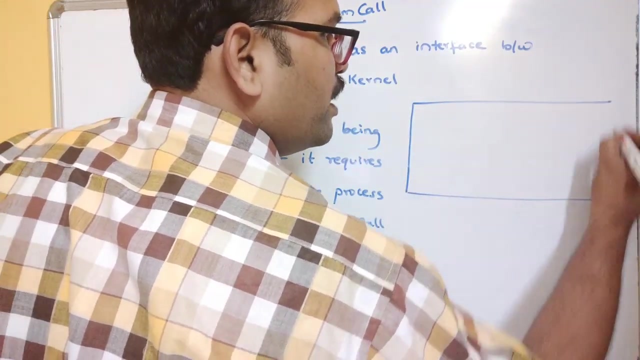 and by execution of this system call the kernel, will give the resource to the process And in the previous session we have already discussed about the memory, different types of memory Right. So the memory is divided into two categories. Memory is divided into two categories. 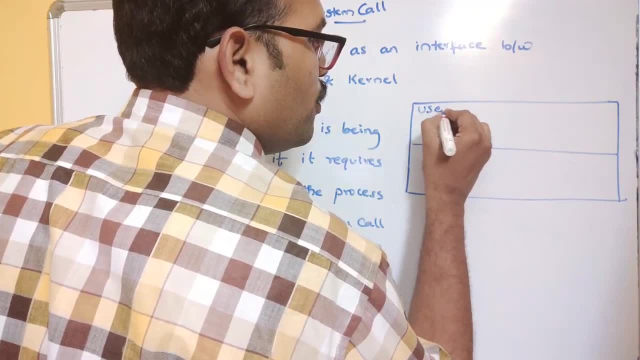 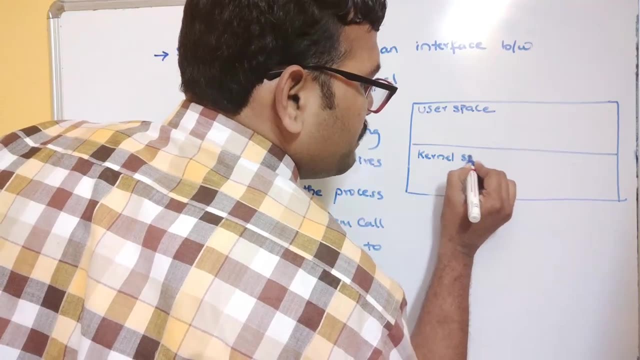 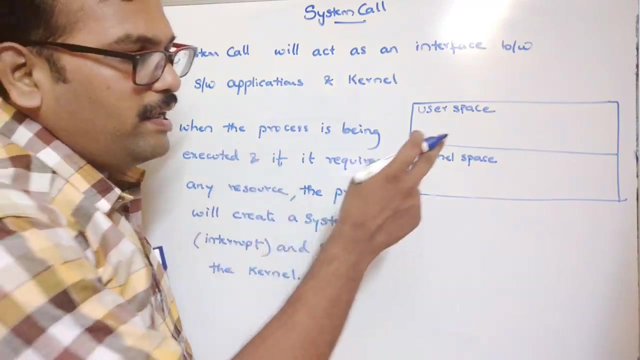 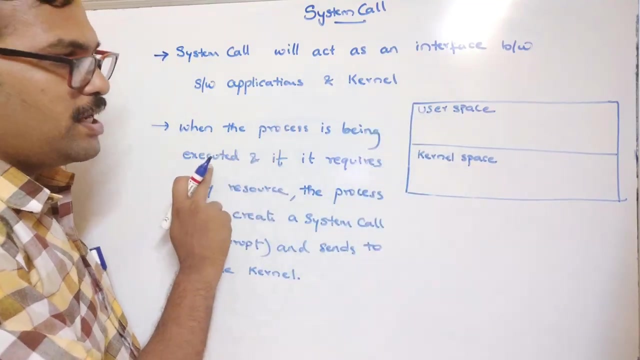 So one is user space and another one is kernel space. Kernel space, Right? So all the system calls will be get executed in the kernel space itself and the system calls will be created in the user space, because the process execution will be in user space. 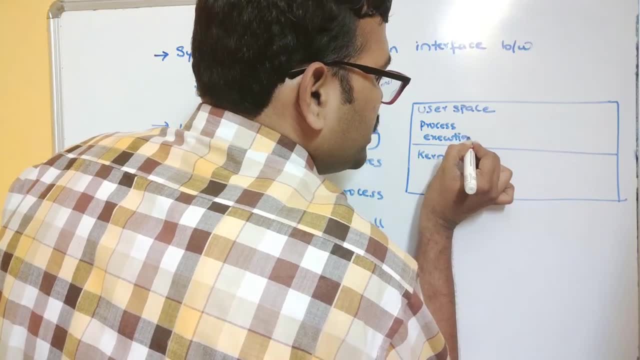 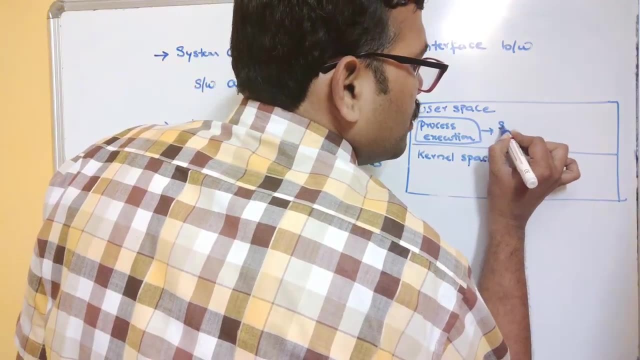 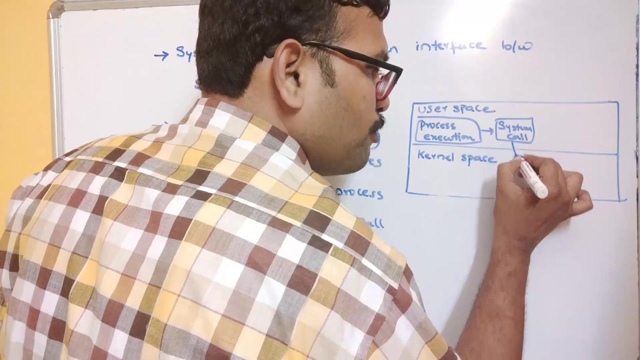 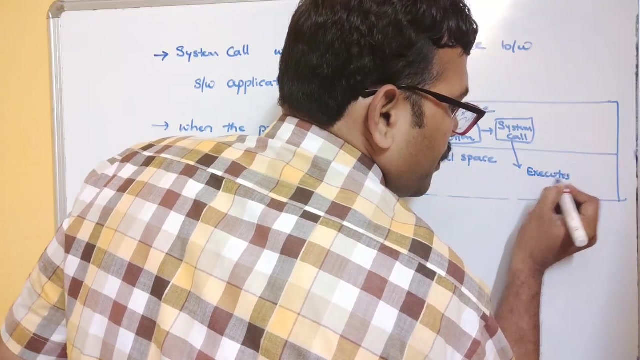 The process execution will be in the user space whenever it requires any resource. immediately a system call will be generated. a system call will be generated and immediately this system call will be sent to the kernel space and here it executes the system call, and the system call will be executed in the kernel space itself. 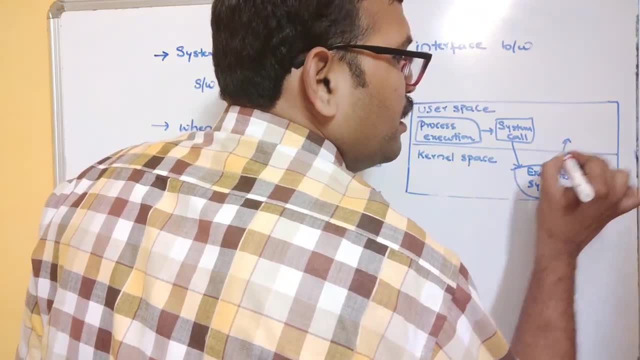 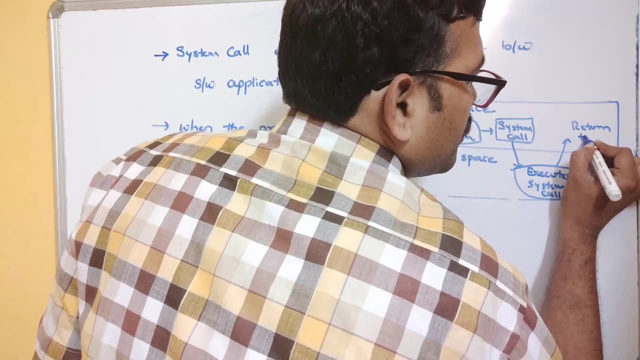 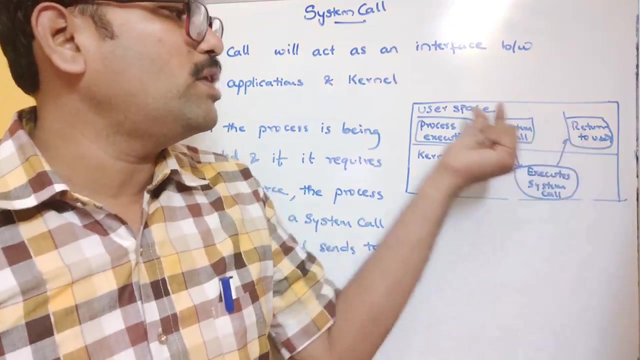 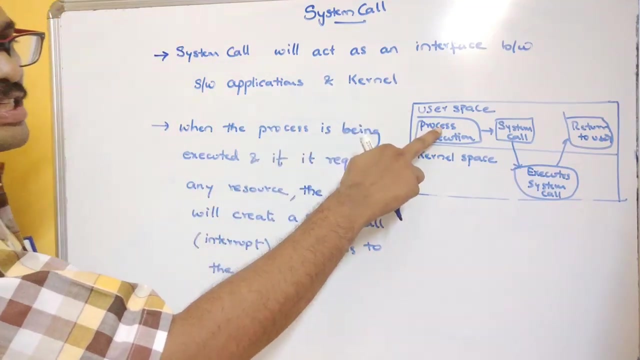 Okay, Okay, And immediately after that, again the control will move back to. So, after completion of execution, automatically the control will move back to the user space and automatically the execution of system call will be being executed. Right. So, whenever the process is being executed in a user space, whenever it requires any 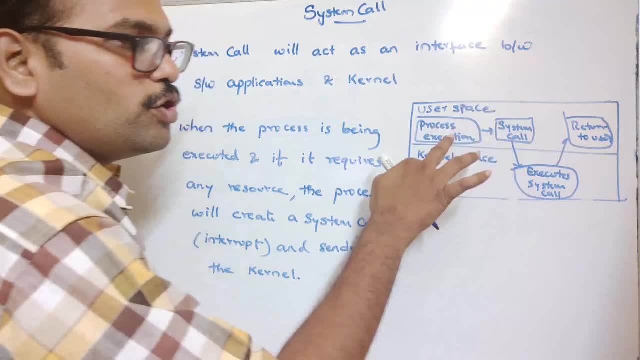 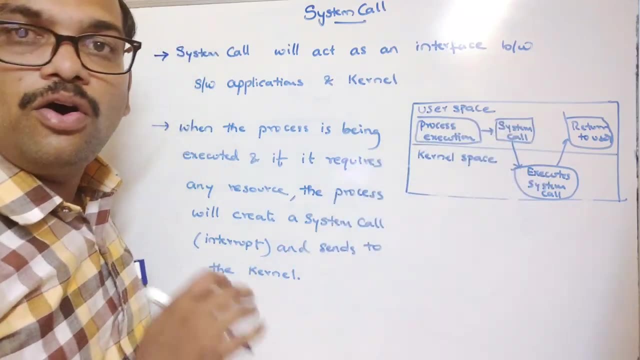 resource immediately it will. So the resource will be provided by the kernel Right. The resource will be provided by the kernel, So it will create a system call or an interrupt. So we can also call it as an interrupt. 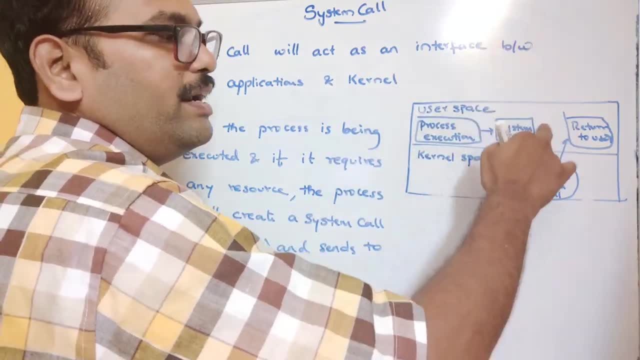 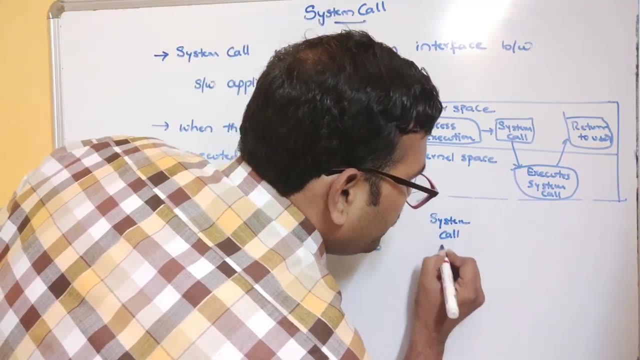 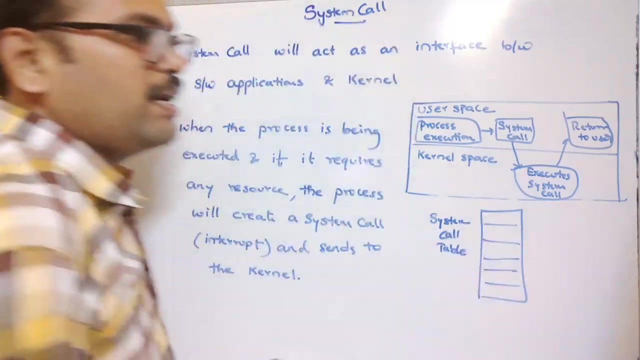 So it will create a system call and through system call it will enter into the kernel space and here a system call table will be maintained. System call table. So in this table it stores all the system calls which are generated by the from the 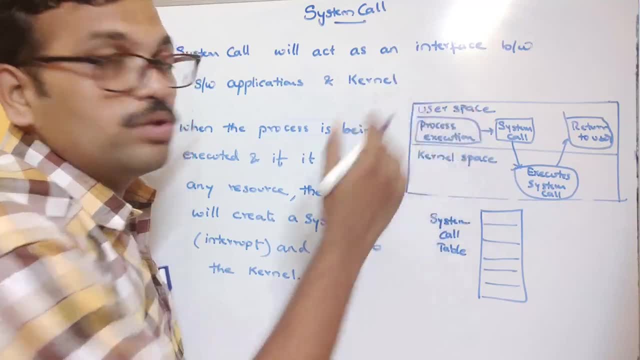 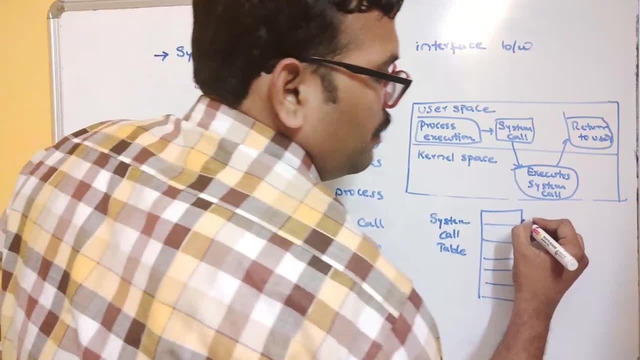 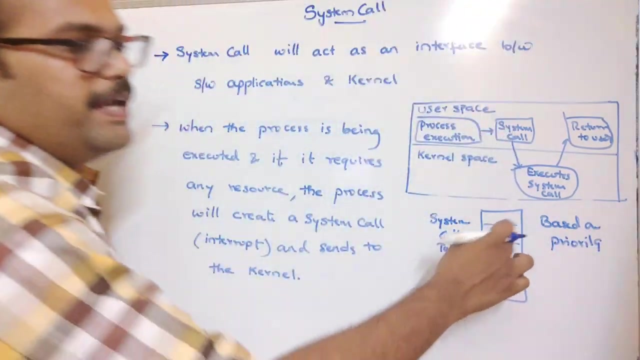 user space, which are entered into the kernel space through the user space, Right? So here we are getting all the system calls here and based on the priority, based on priority, each system call will be get executed and immediately the control will go back to the 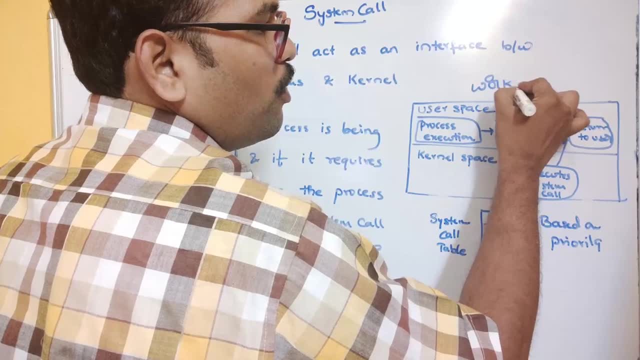 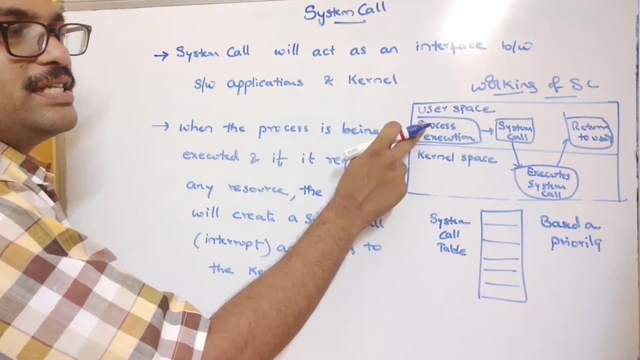 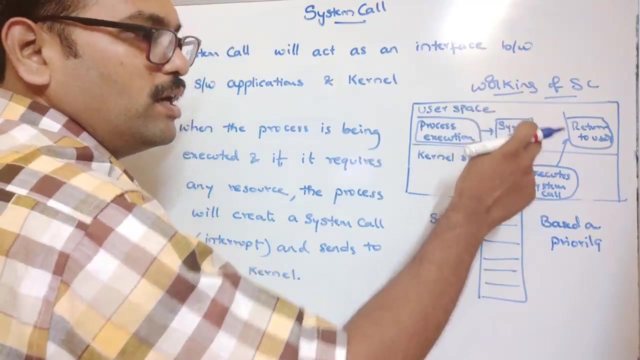 user space. So this is the working of system call, Working of system call Right. So whenever the process is executed in the user space, if it requires any resource, immediately the system call will be generated and through that it will enter into the kernel. 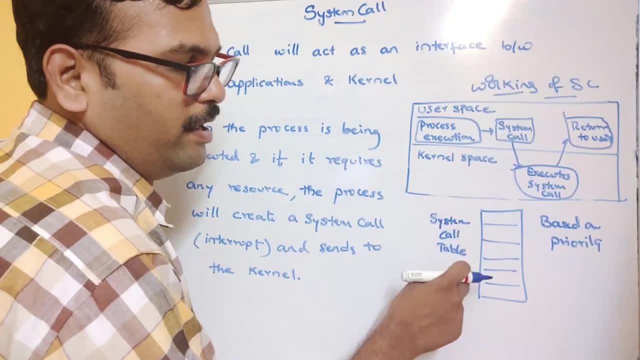 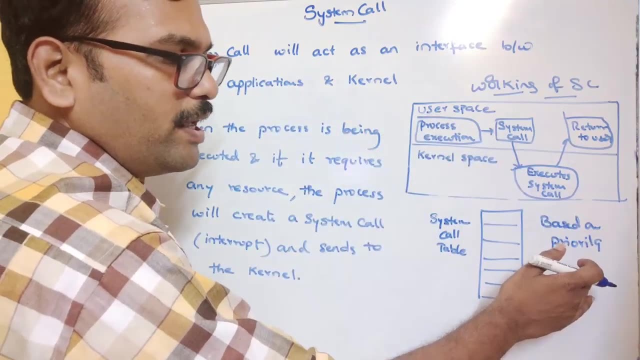 space and in the kernel space, a system call table will be maintained and in this system call table the address of each and every system call will be maintained and, based upon the priority, one by one, the system call will be retrieved from this table and that 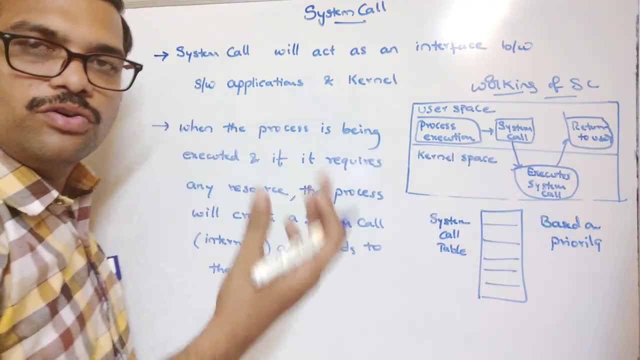 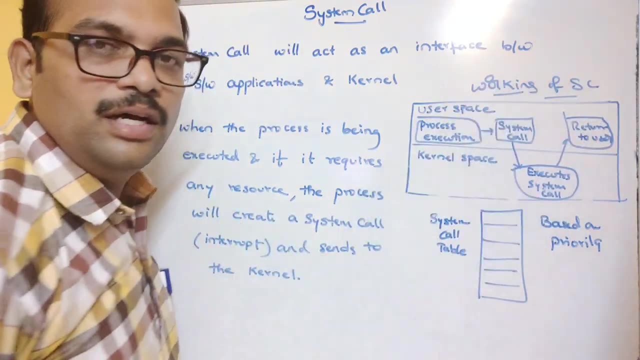 system call will be executed and the I mean the resource resource retrieval, The resource retrieval will be required will be given to the process and the control will get back to the user space. So this is the working of any system call. 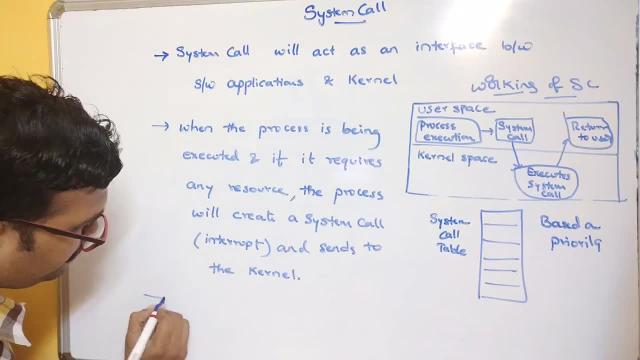 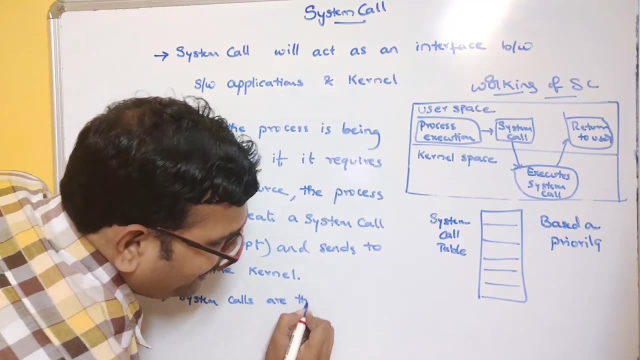 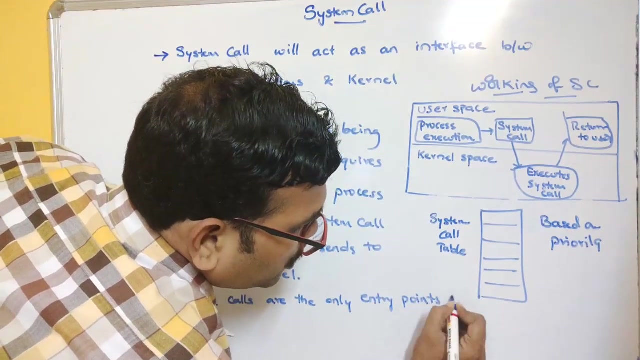 Right. So one point, that is, system calls are the only entry points, only entry points to kernel space, Right, Okay, So the? so every time we call an application, we call an application to the kernel space and these are the only entry points. 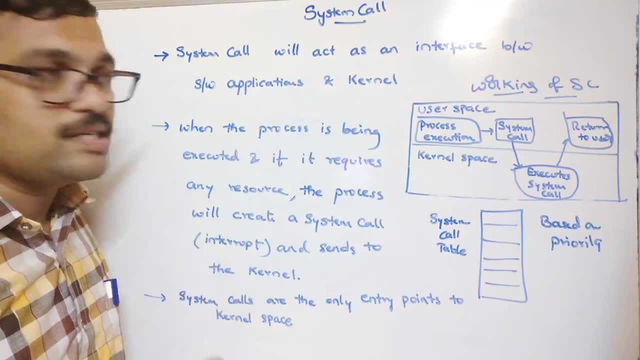 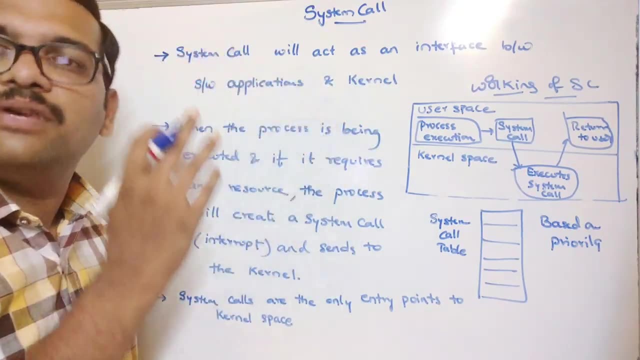 That means in the previous sessions we have discussed about the kernel and kernel services, right? So in that we have discussed about this one, the two modes, one is a user space and other one is a kernel space. And we call this kernel space as a protected kernel space, so that no other application 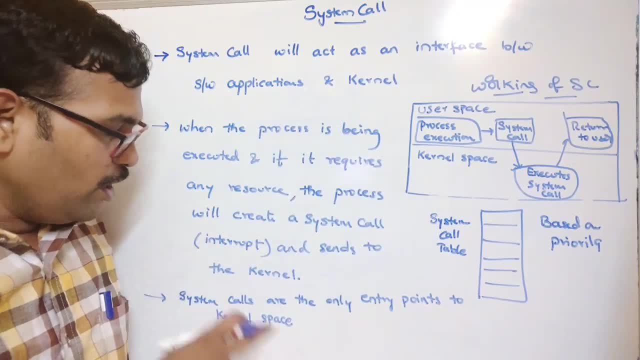 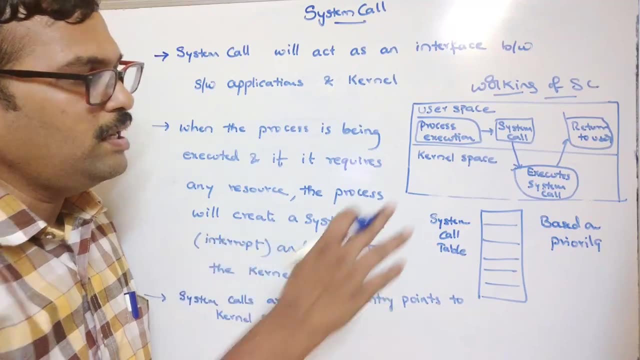 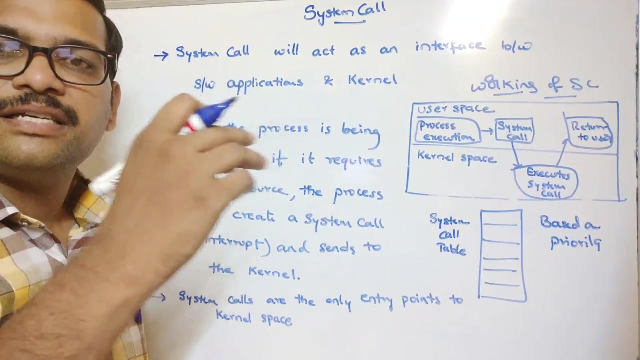 will get access into this kernel space. So that's why only the system calls are the entry points to the kernel space. Okay, So no other application can enter into the kernel space, right? So these are the system calls. A system call is an interface between the application and the kernel.